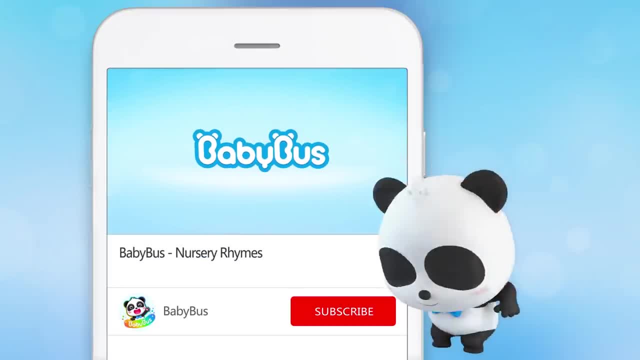 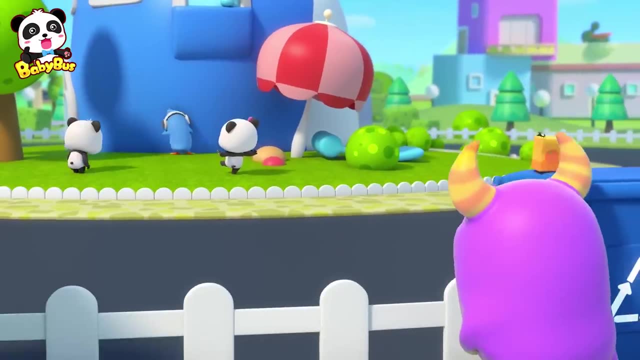 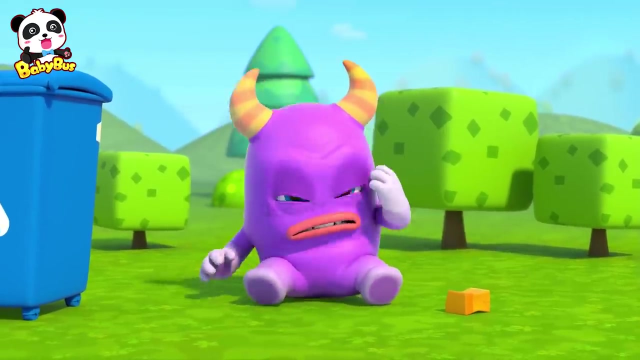 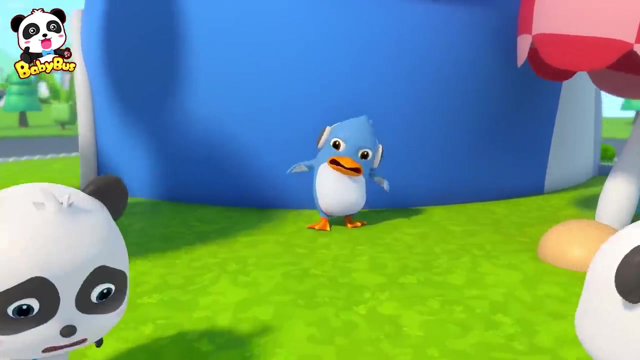 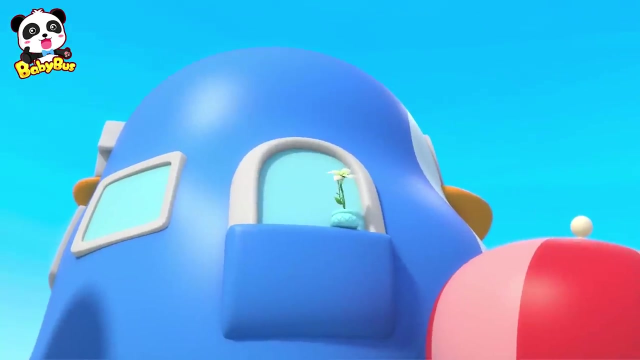 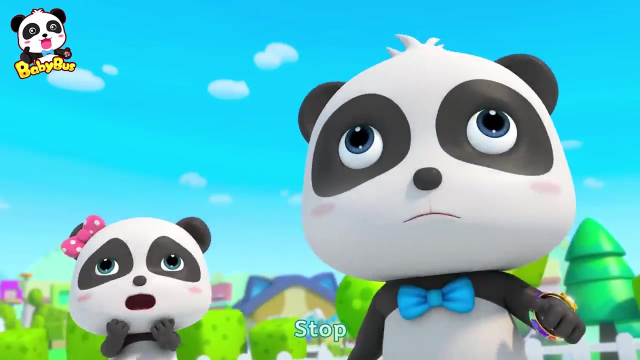 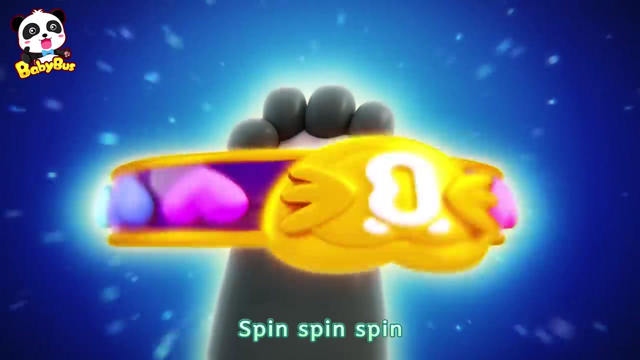 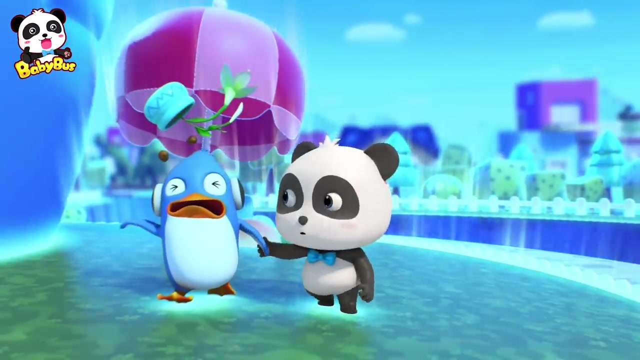 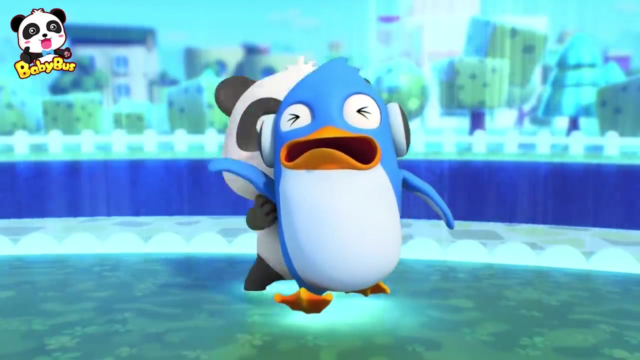 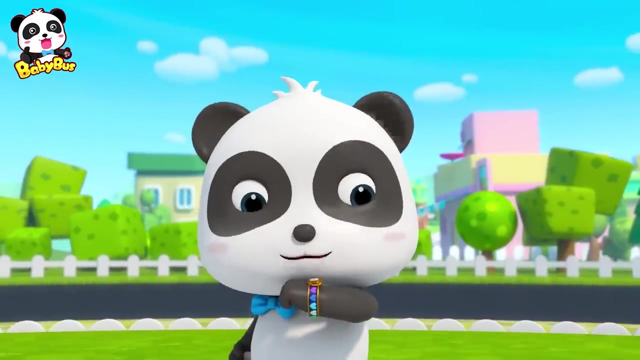 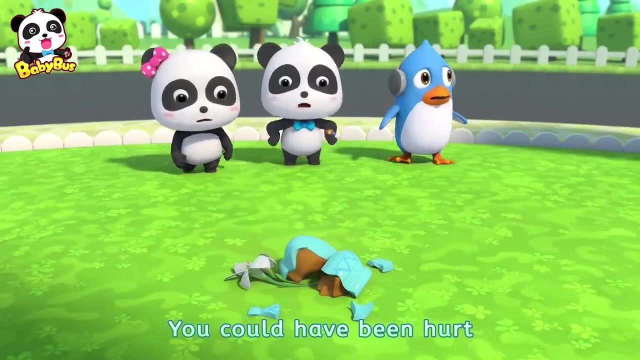 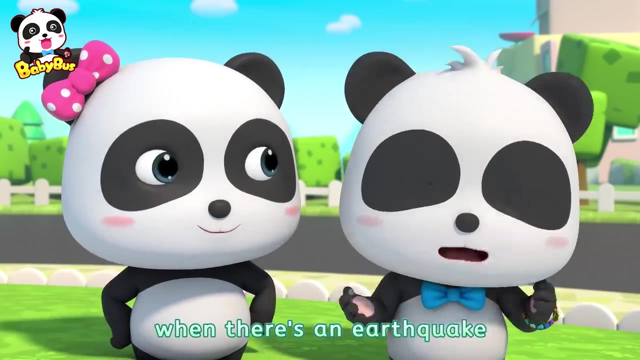 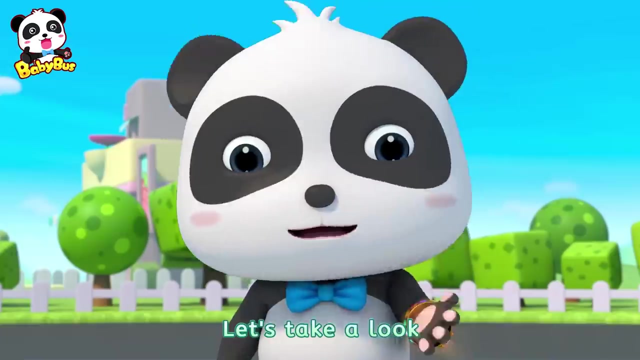 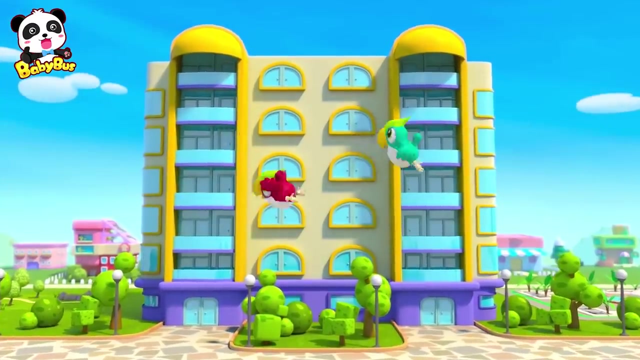 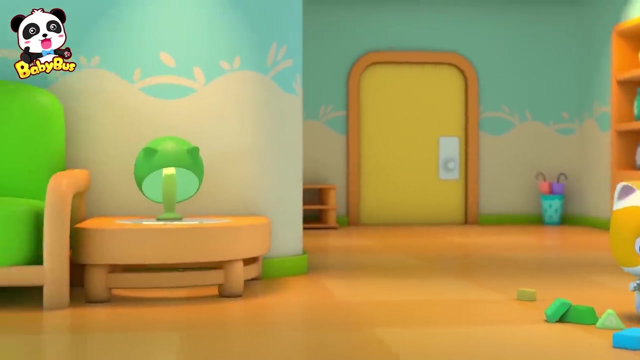 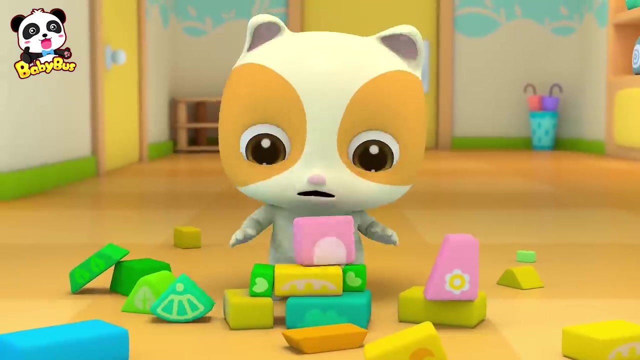 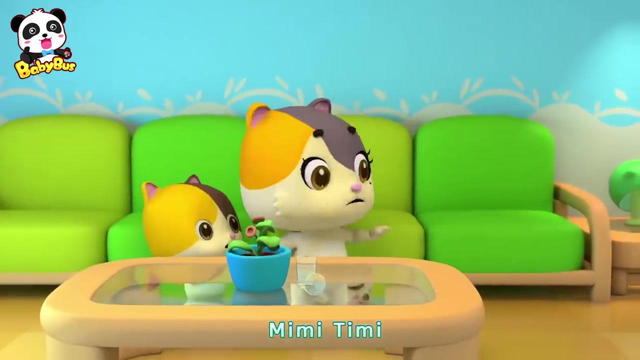 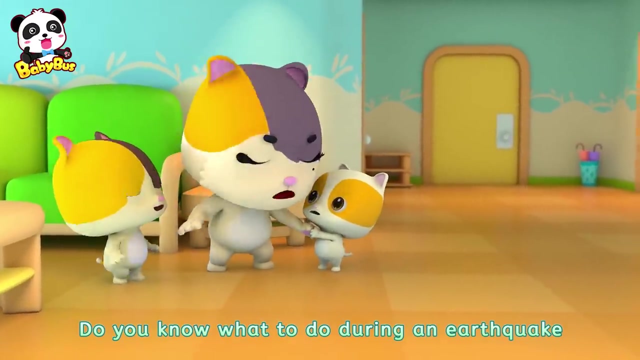 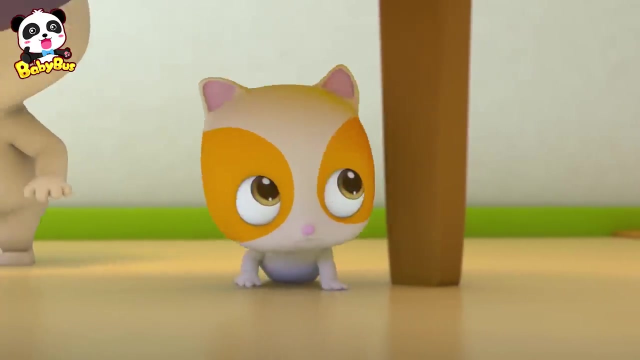 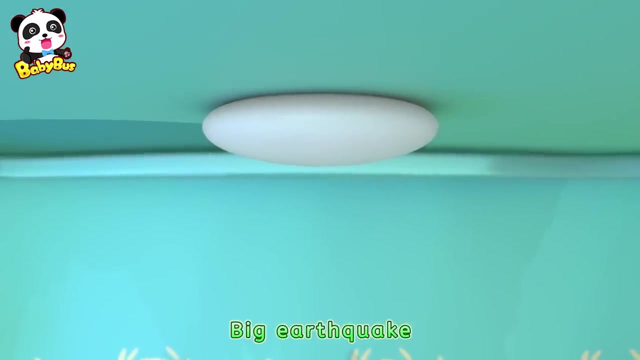 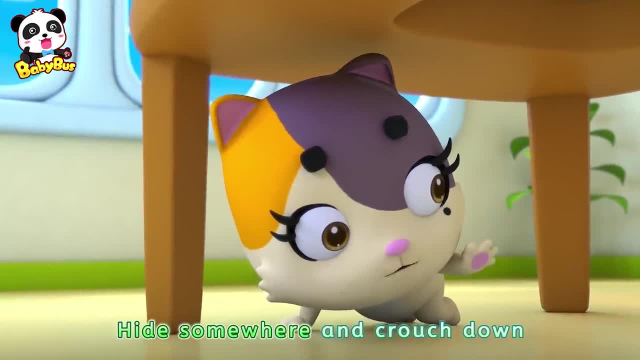 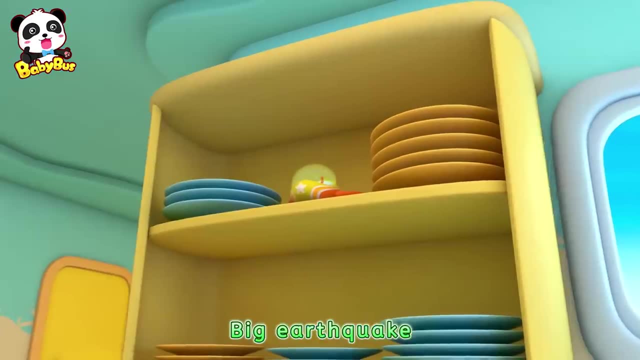 Dangerous, dangerous. Stay calm, please hide somewhere and crouch down. Hold on tight with your hands. You must do this to be safe, To be safe. Big earthquake: shaking, shaking, Big earthquake, shaking, shaking, Big earthquake, dangerous, Shaking, shaking, dangerous. 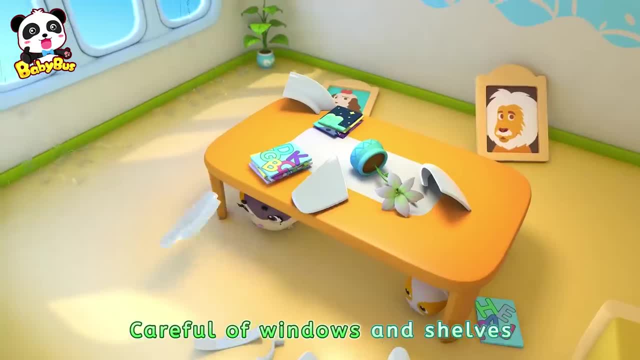 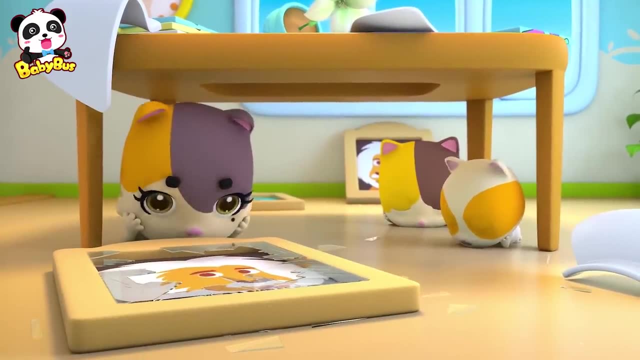 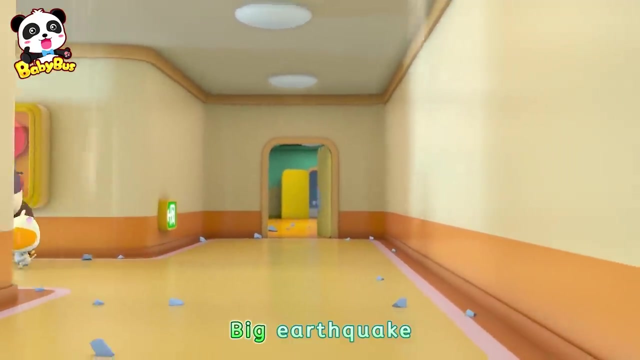 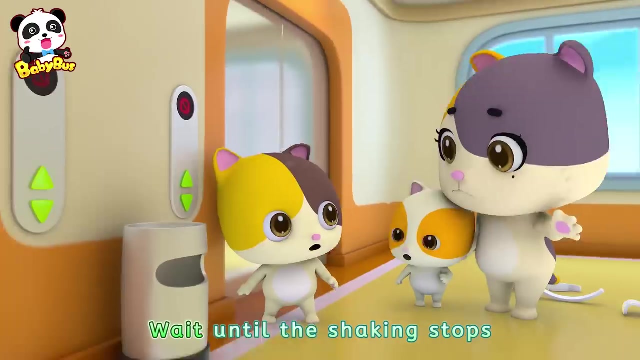 Dangerous. Stay calm, please careful of windows and shelves. Please stay in a safe place. You must do this to be safe, To be safe. Big earthquake, shaking, shaking, Big earthquake, big earthquake, Dangerous, shaking, shaking, Dangerous, dangerous. Mario, Stay calm. please wait until the shaking stops. 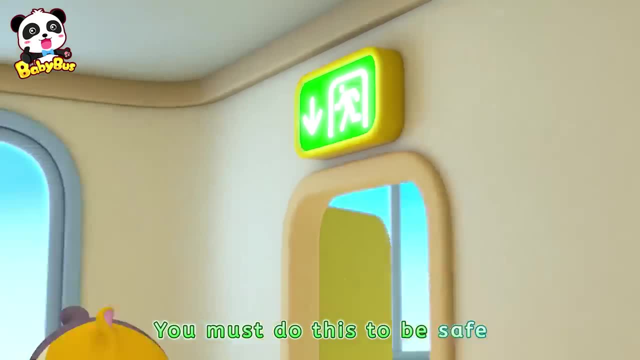 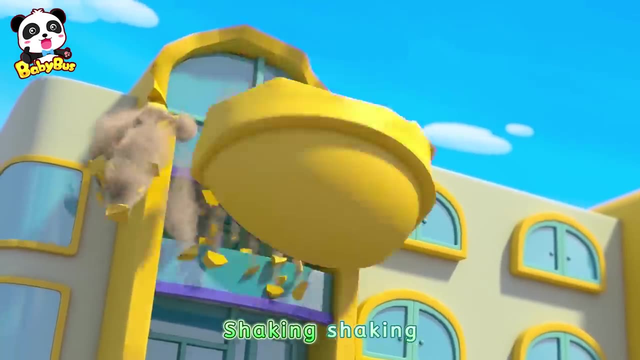 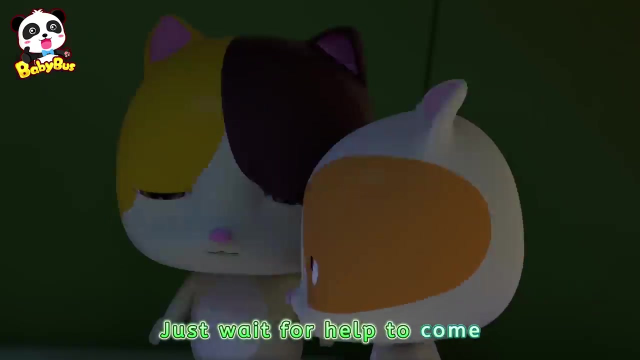 Do not use the elevator. you must do this to be safe, To be safe. Big earthquake- shaking, shaking, Big earthquake, big earthquake, Dangerous, shaking, shaking, Dangerous, dangerous. Stay calm, please. you don't need to cry and shout, Just wait for help to come. 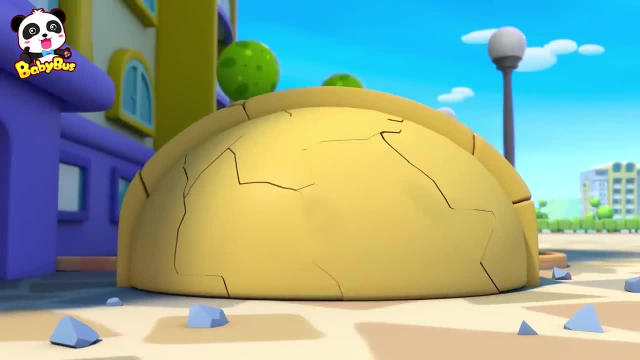 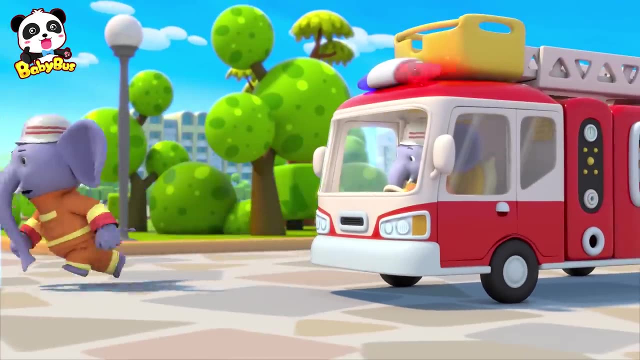 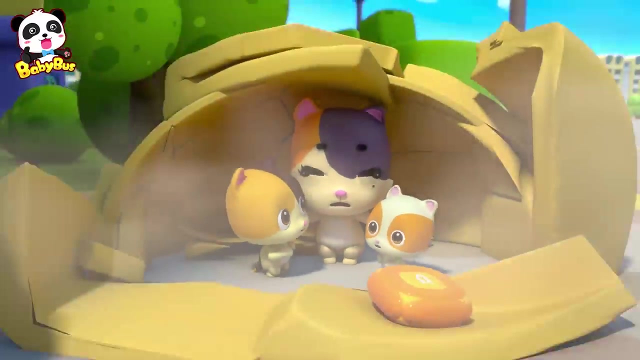 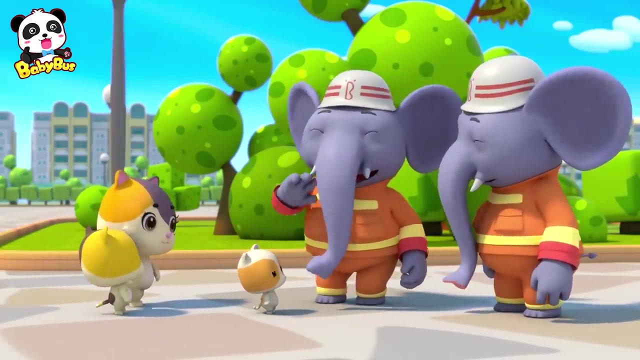 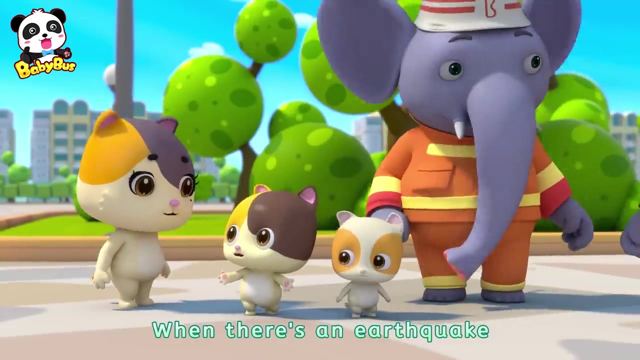 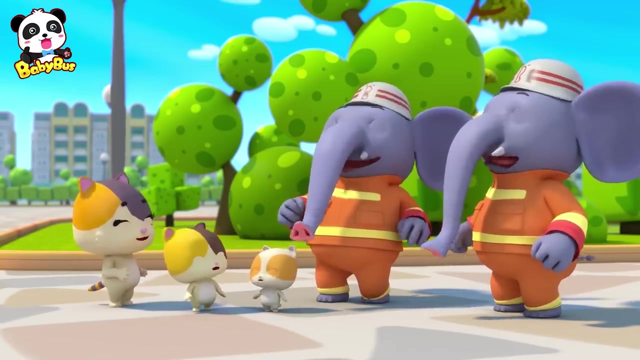 You must do this to be safe, To be safe. Please be safe. Please be safe. Is everyone okay? Thank you, firefighter elephant. You're welcome. You did a great job. today, When there's an earthquake, we need to protect ourselves. You're right. Excellent, Thank you, I got it. 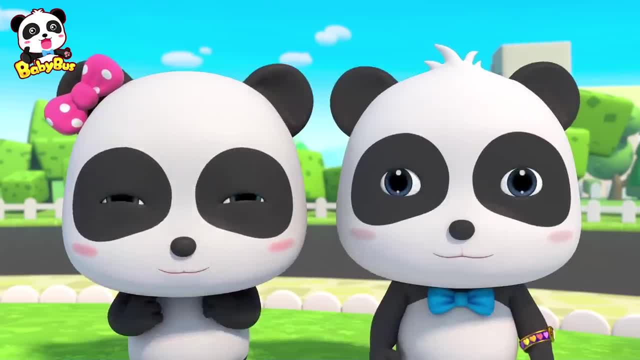 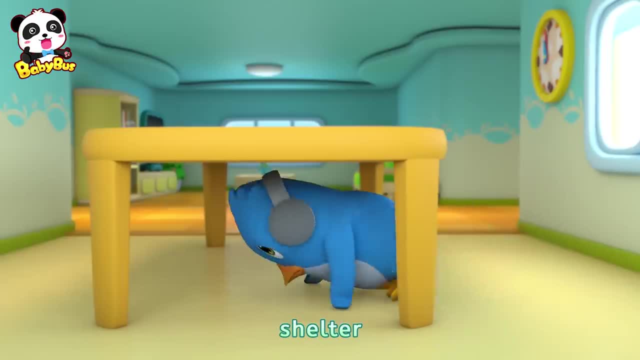 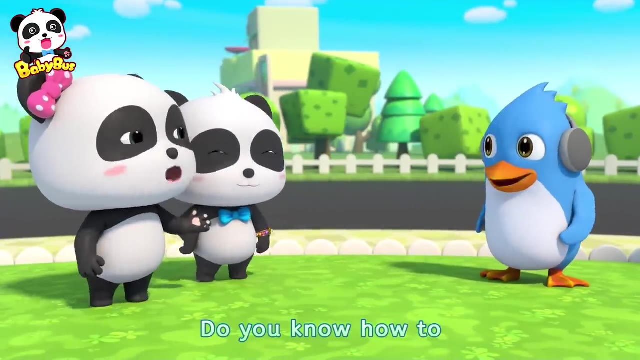 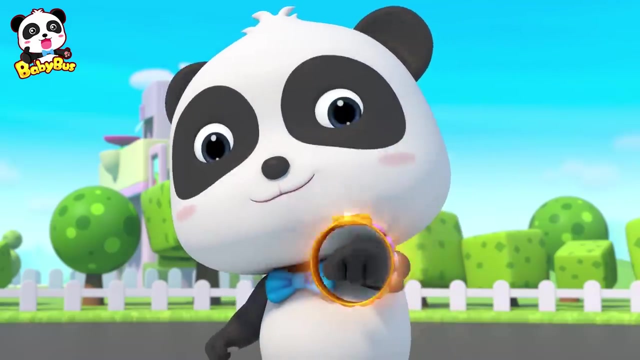 We need to crouch down to protect ourselves And remember the tips: Crouch shelter and stay calm. Crouch shelter and stay calm. Do you know how to prepare for earthquakes? Let's take a look. Make sure you have a mask. Make sure that furniture is safely fixed to the wall. 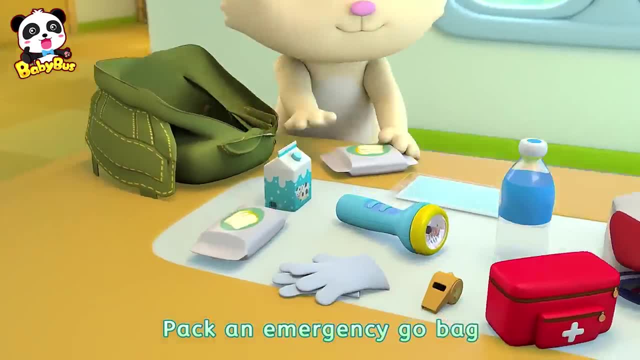 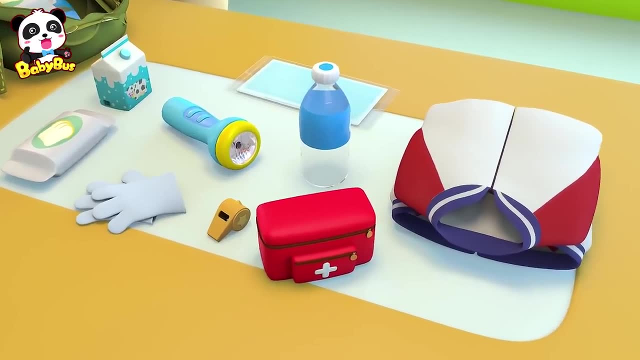 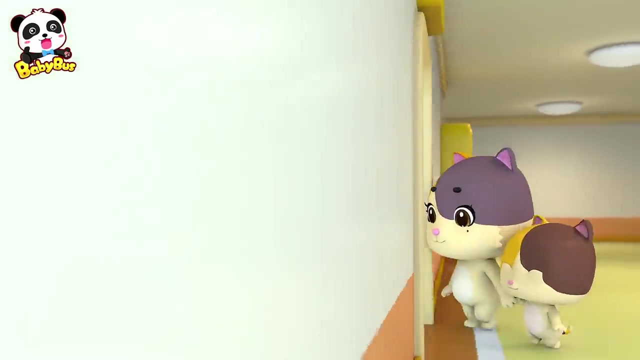 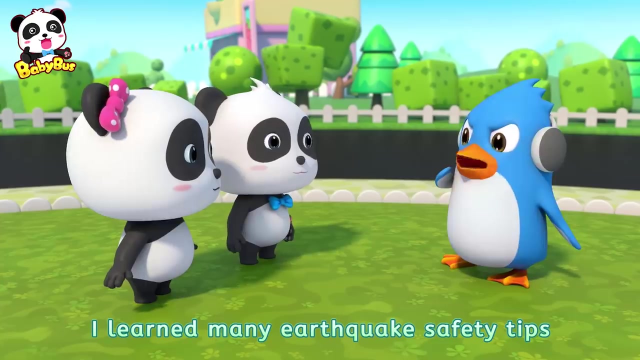 So that they won't fall over. Pack an emergency go bag, Put in some water, food, masks, a flashlight, gloves, a whistle, a jacket and a first aid kit And check the locations of the emergency exits. Thanks guys, I learned many earthquake safety tips. 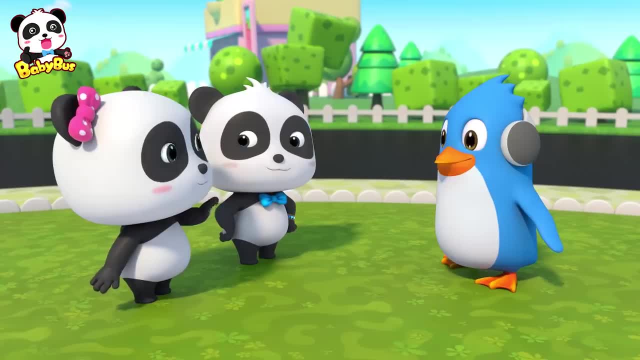 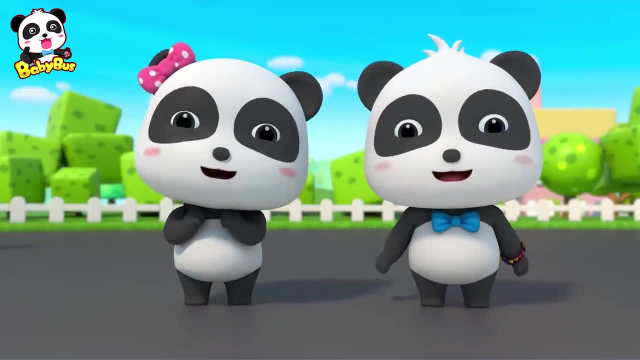 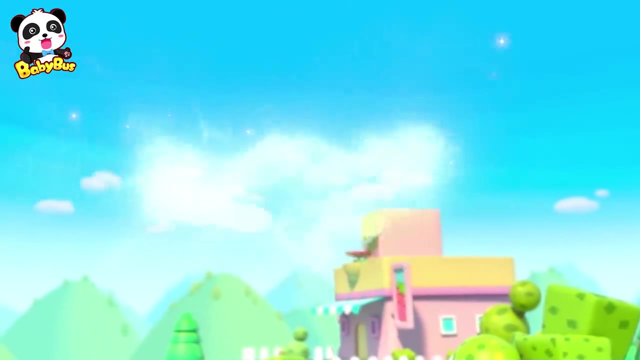 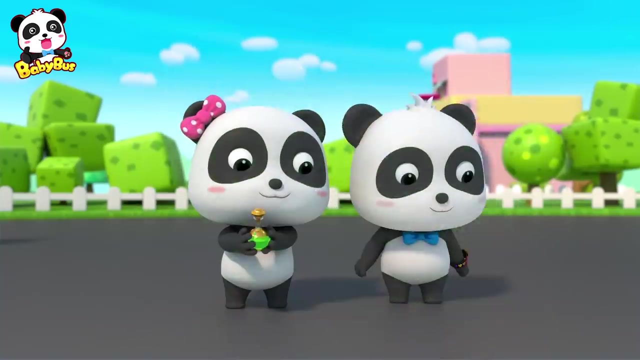 So I think I can protect myself. You're welcome, Kids, do you remember what we've learned today? Great, You've learned about safety. Wow, Wow, Yay, We've got a bottle of magic potion. Oh, no, They've got a magic potion. We've got a magic potion.